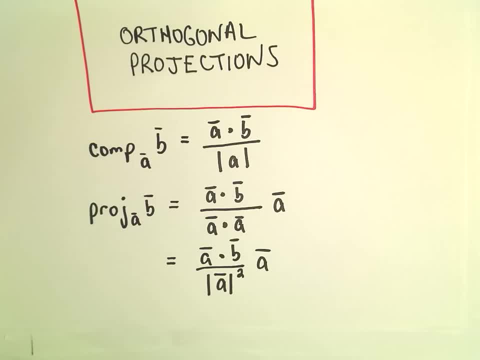 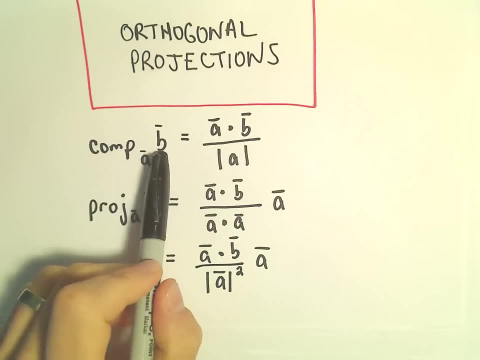 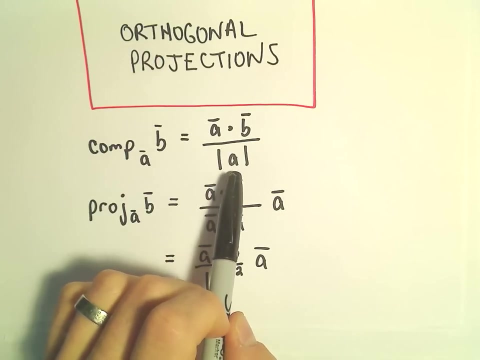 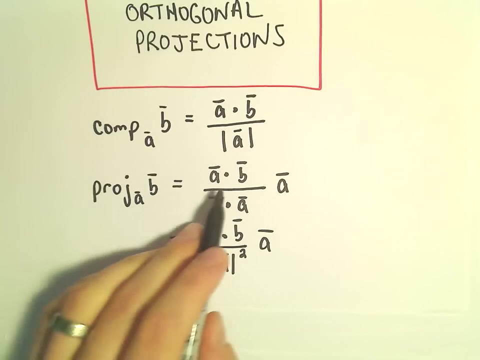 All right. in this video we're going to look at finding components of vectors along another vector and projections of vectors onto other vectors. So to figure out the component of B onto A, we take the dot product A, dot B and we divide that by the magnitude of vector A. And then to figure out the projection of vector B along vector A, we take A, dot B over A dot A and multiply that by vector A. 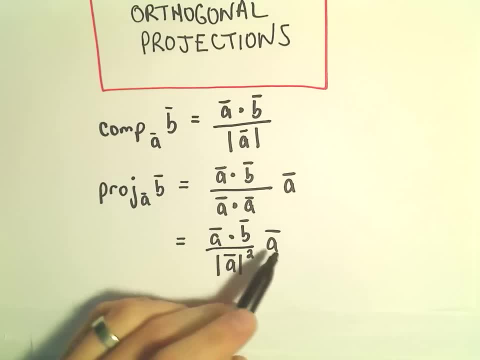 Equivalently we can write that as A dot B over the magnitude of A, squared again times vector A. So if I leave off any of the little lines, again those indicate vectors. Everything I'm talking about here is vectors, so hopefully I won't accidentally do that. 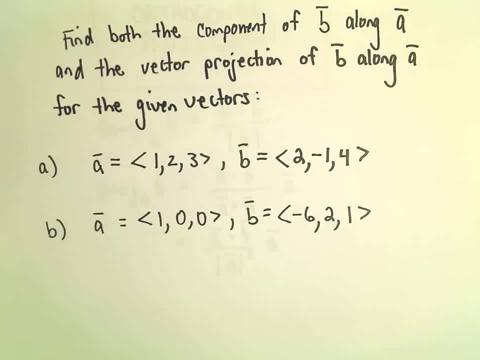 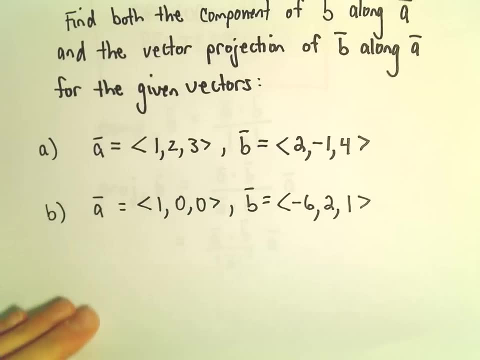 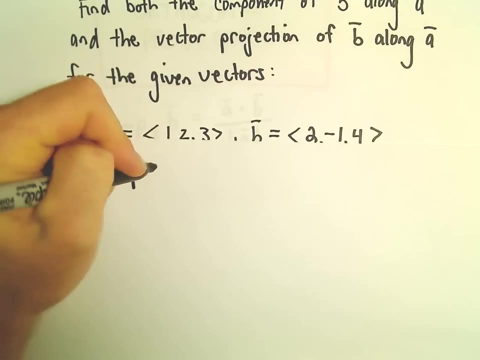 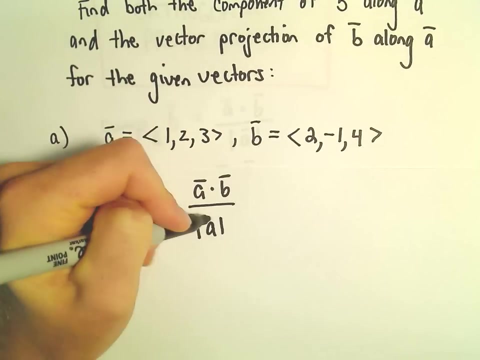 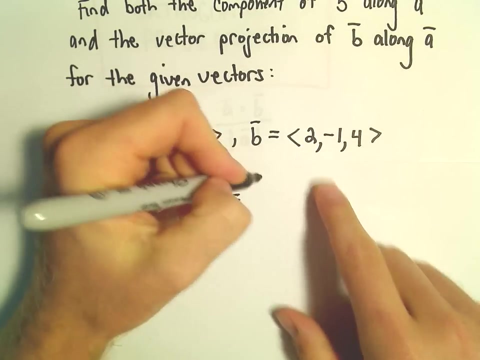 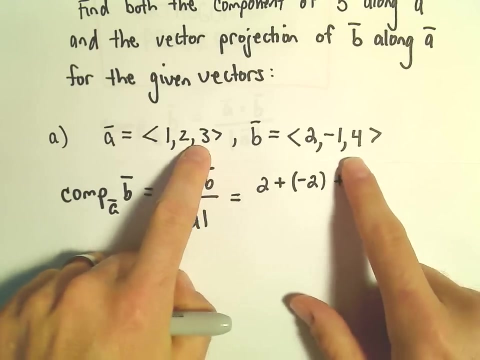 Okay, so what we want to do is we're going to find both the component of B along A and also the vector projection of B along A for these given vectors. All right, so again to do the component, so to figure out the component of vector B along A, again we take the dot product A, dot B, and then we divide that by the magnitude of vector A, So to do the dot product. again, we just multiply respective components. So 1 times 2 will be 2.. We'll take 2 times negative 1, that'll be negative 2.. Then we'll add to that 3 times 4, which is going to be 12.. 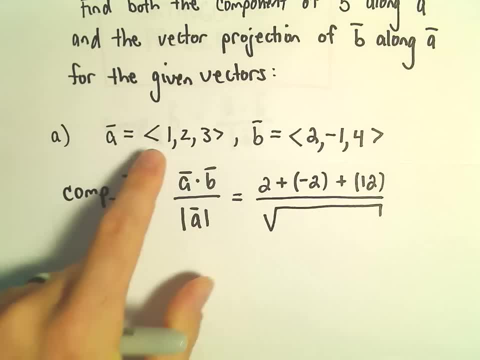 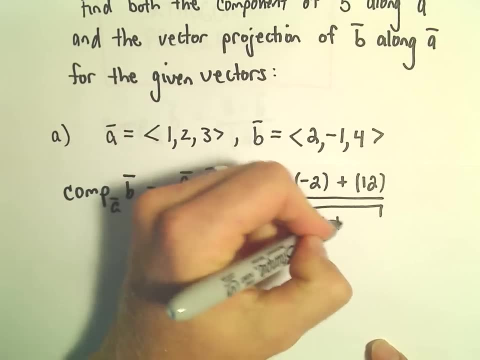 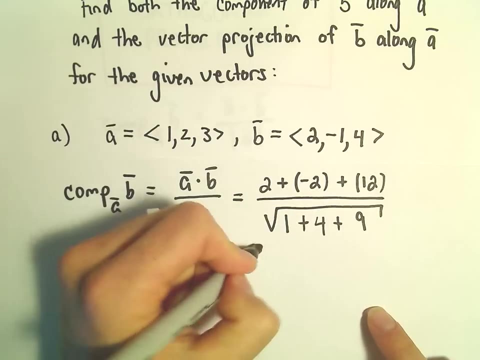 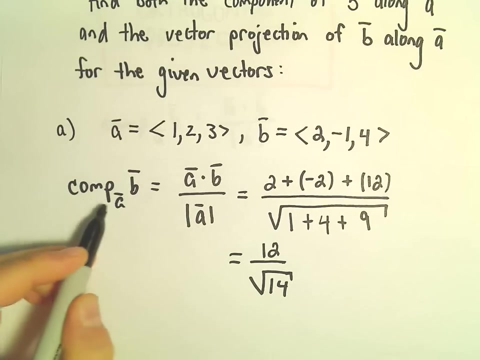 We'll divide that by the magnitude of vector A. Well, the magnitude, we just square the components. so 1 squared is 1,, 2 squared is 4, 3 squared is going to be 9.. And now we can just simplify this. So 2 plus negative 2 is 0, we'll have 12 on top In the denominator. it looks like we're going to have the square root of 14.. So that's our component of vector B along vector A To do the projection. 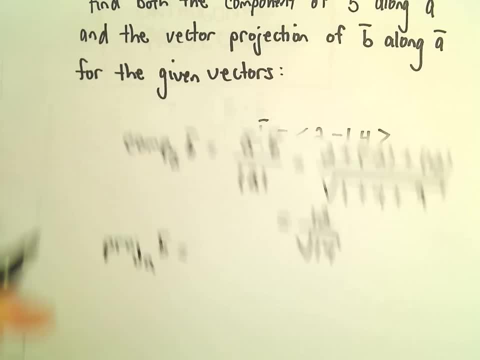 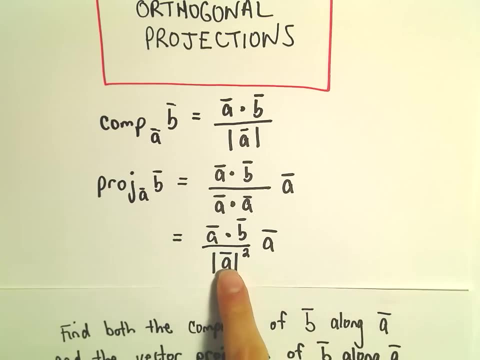 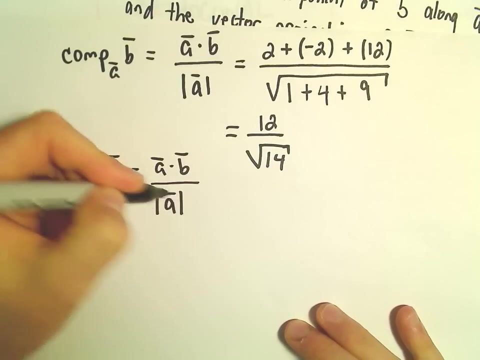 the projection of B along A. Again, the formula for that we just said was A dot B, and I'm going to use this slightly different. instead of doing A dot A, I'm going to take the magnitude squared, because we've already figured out the magnitude, and then we'll multiply that. 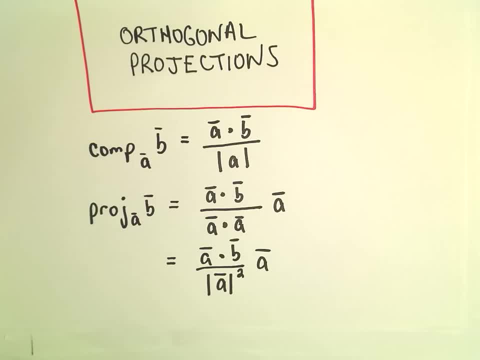 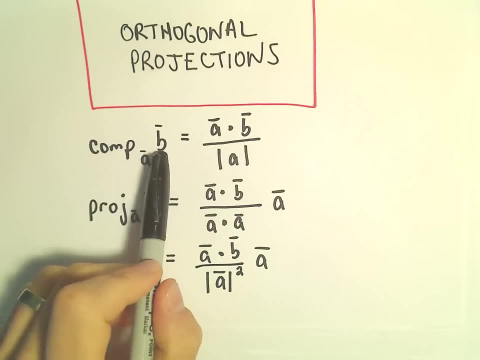 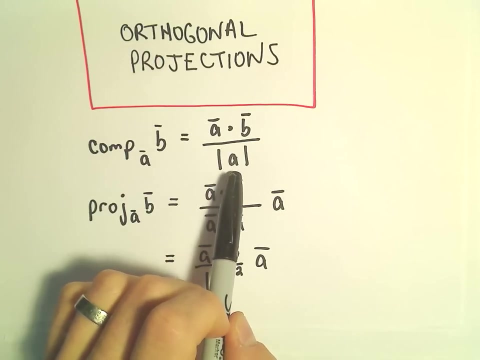 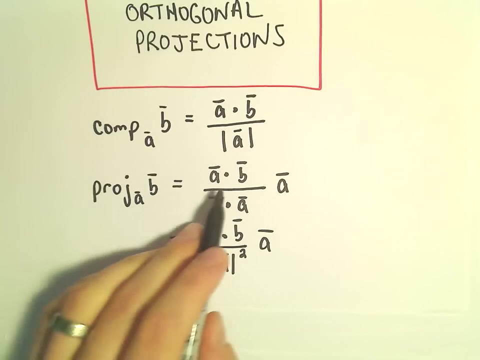 All right. in this video we're going to look at finding components of vectors along another vector and projections of vectors onto other vectors. So to figure out the component of B onto A, we take the dot product A, dot B and we divide that by the magnitude of vector A. And then to figure out the projection of vector B along vector A, we take A, dot B over A dot A and multiply that by vector A. 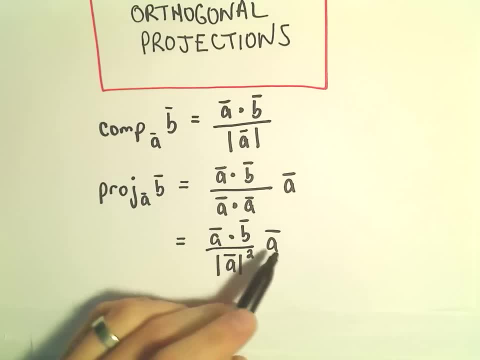 Equivalently we can write that as A dot B over the magnitude of A, squared again times vector A. So if I leave off any of the little lines, again those indicate vectors. Everything I'm talking about here is vectors, so hopefully I won't accidentally do that. 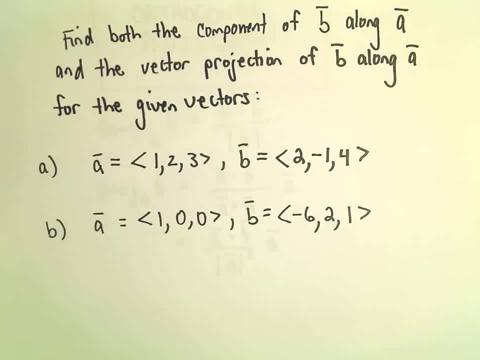 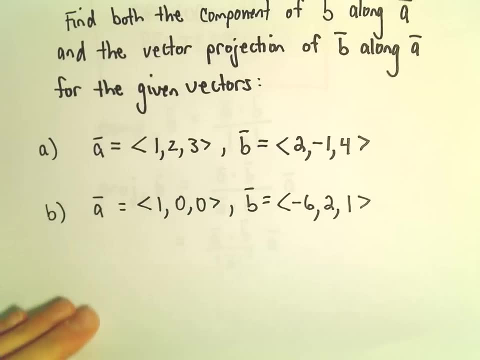 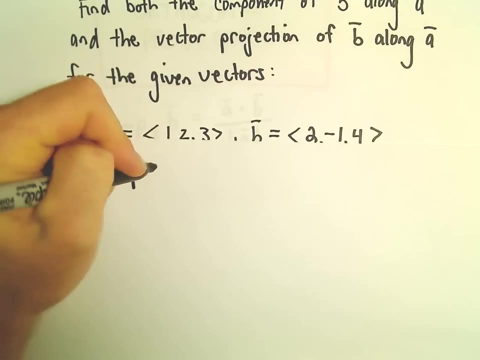 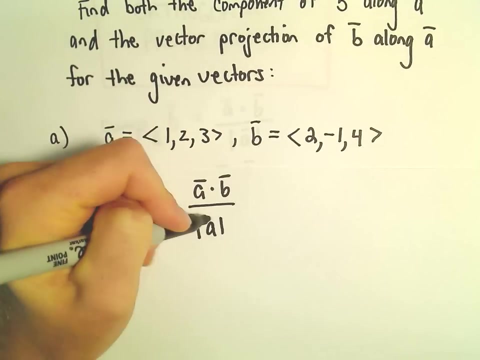 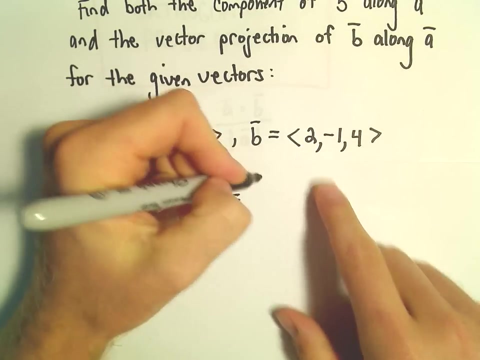 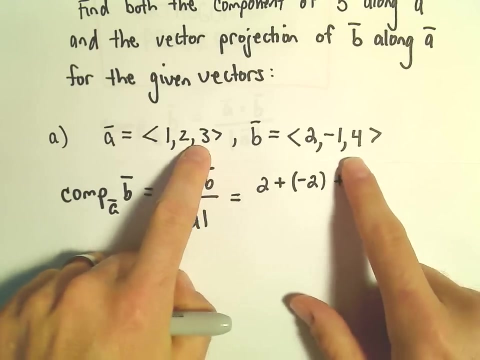 Okay, so what we want to do is we're going to find both the component of B along A and also the vector projection of B along A for these given vectors. All right, so again to do the component, so to figure out the component of vector B along A, again we take the dot product A, dot B, and then we divide that by the magnitude of vector A, So to do the dot product. again, we just multiply respective components. So 1 times 2 will be 2.. We'll take 2 times negative 1, that'll be negative 2.. Then we'll add to that 3 times 4, which is going to be 12.. 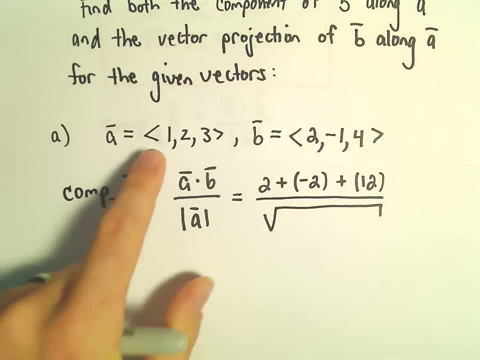 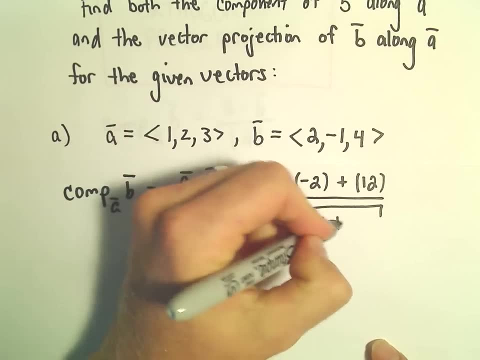 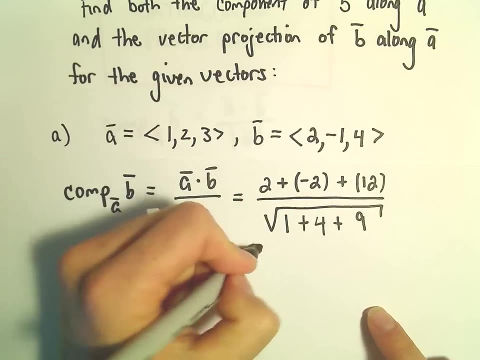 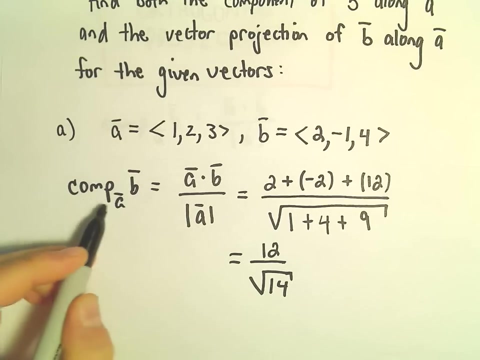 We'll divide that by the magnitude of vector A. Well, the magnitude, we just square the components. So 1 squared is 1,, 2 squared is 4, 3 squared is going to be 9.. And now we can just simplify this. So 2 plus negative 2 is 0, we'll have 12 on top In the denominator. it looks like we're going to have the square root of 14.. So that's our component of vector B along vector A To do the projection. 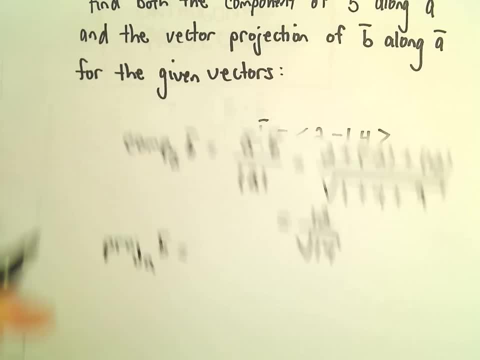 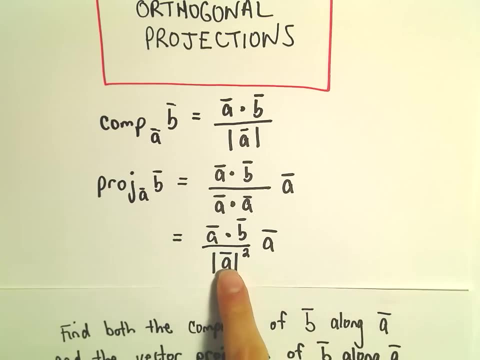 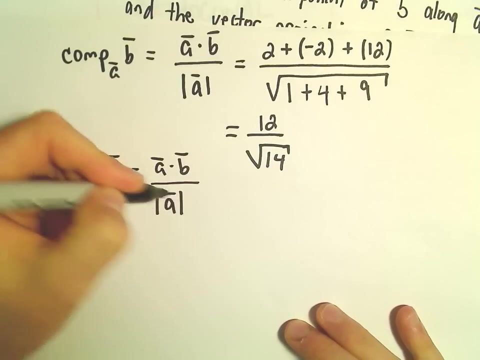 the projection of B along A. Again, the formula for that we just said was A dot B, and I'm going to use this slightly different. instead of doing A dot A, I'm going to take the magnitude squared, because we've already figured out the magnitude, and then we'll multiply that.